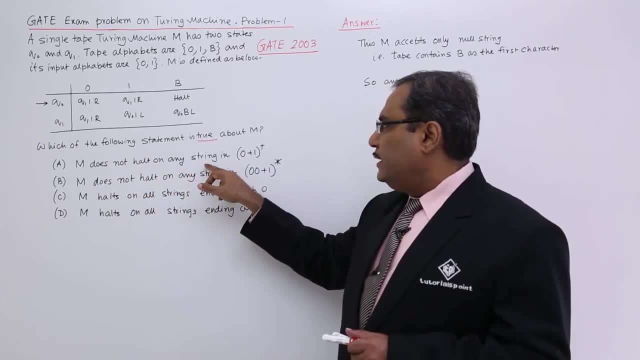 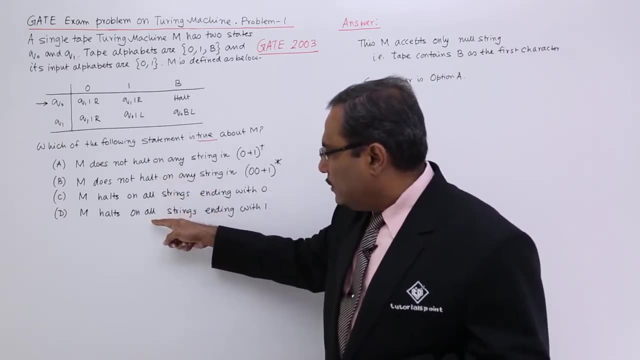 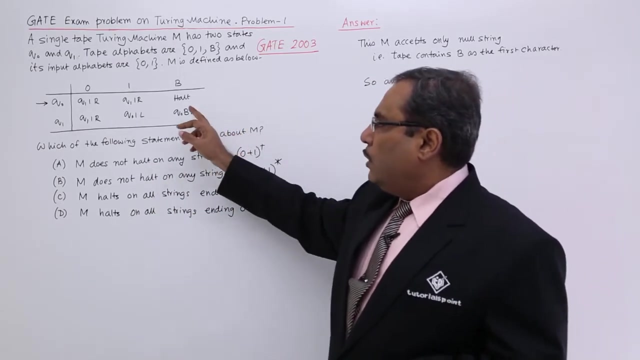 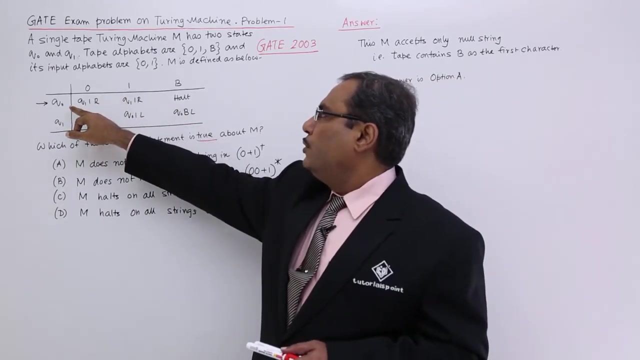 by one. So M does not halt on any string in 0 plus 1 whole plus. Now they are asking the question on halting: It will halt or it will not halt. So here you see, the Turing machine will halt only for Q0B, because at Q1B also it is going to Q0, and then it is. 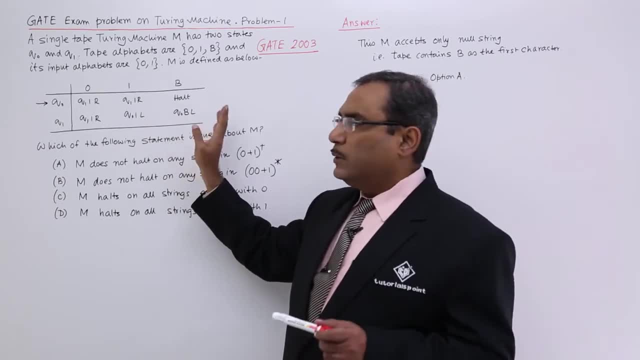 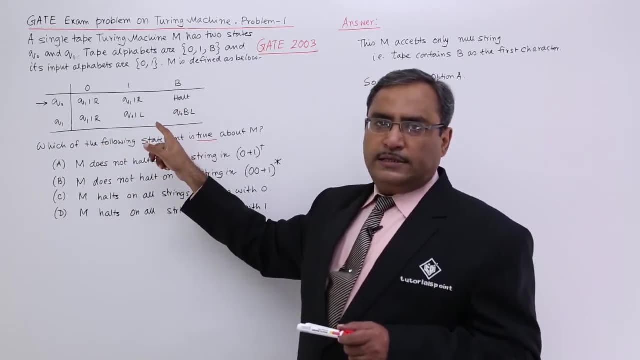 over, adding B by B, and then it is going towards the left, Whatever has been mentioned. So now the thing is that the machine, this particular Turing machine M, is halting only on when we are at the state Q0 and the tape symbol is: 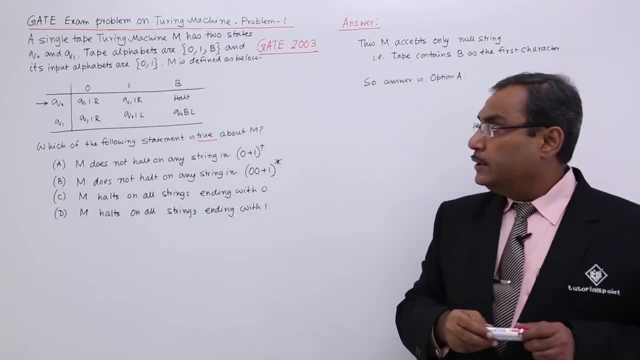 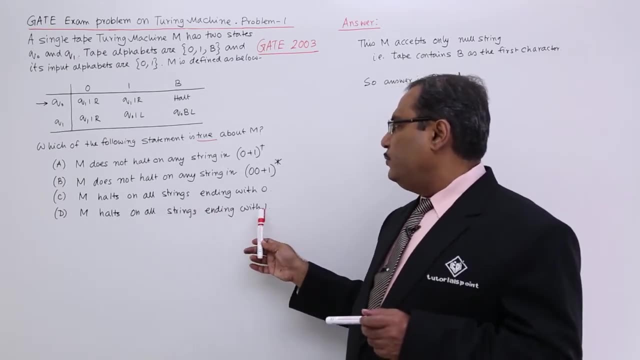 B. So that is in those, in that case only, and otherwise it will not halt. Now see, it halts on the string ending with 1.. In the 1 column there is no question of halting. So this state Q0B is halting. So this is the state. Q0B is halting. So this is the state. 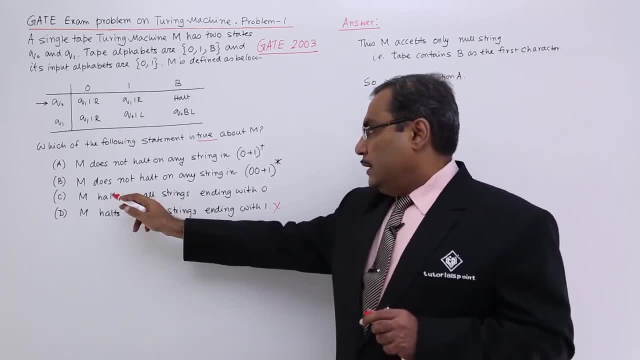 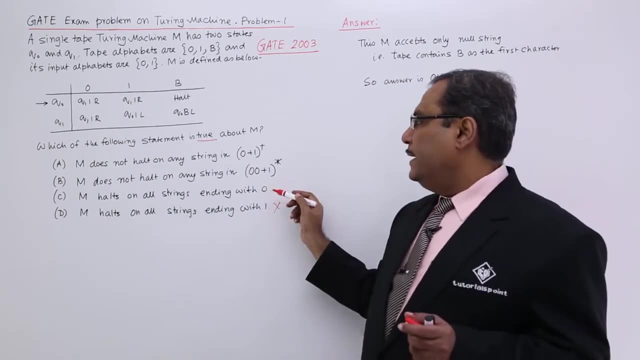 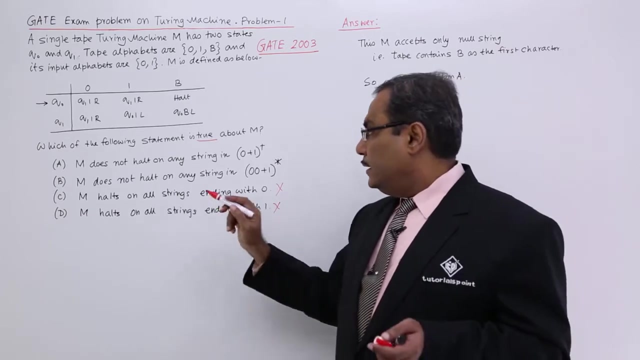 statement is not correct. It halts on all strings ending with 0.. In the 0 column I am not finding any halt. So that is why, ending with 0, the machine will halt. Turing machine M will halt. This is not correct. Now. M does not halt any string in 0 comma. 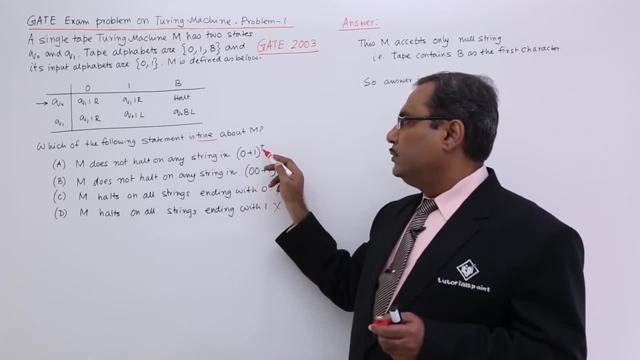 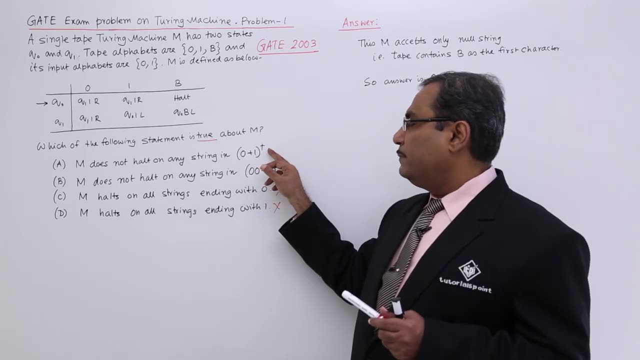 0 plus 1 whole plus. It does not halt. So here you see, here in this case. So this is the state Q0B. We are having this 0 plus 1 whole plus. That means we are having string. 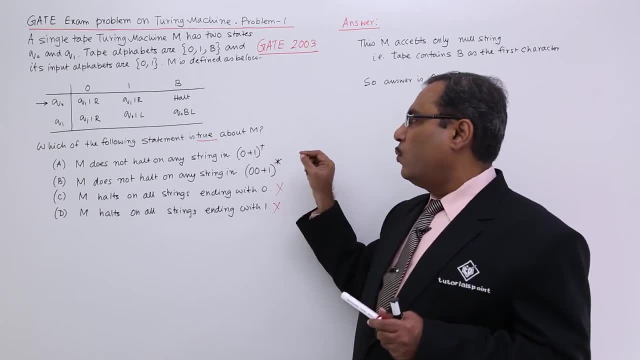 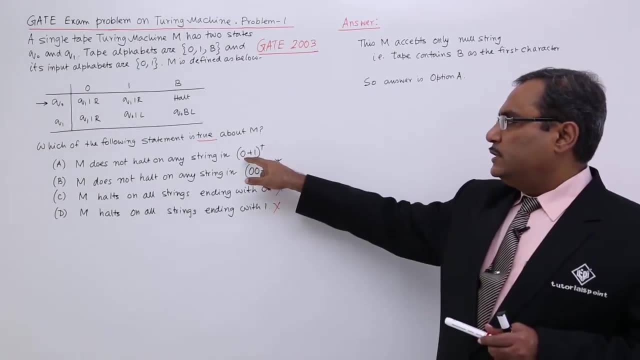 with 0 or 1, or 0, 0, 0, 1, 1, 0, 1, 1.. That means all possible combinations of 0s and 1s. Now see So this particular string, this particular 0 plus 1, whole plus, it cannot produce any. 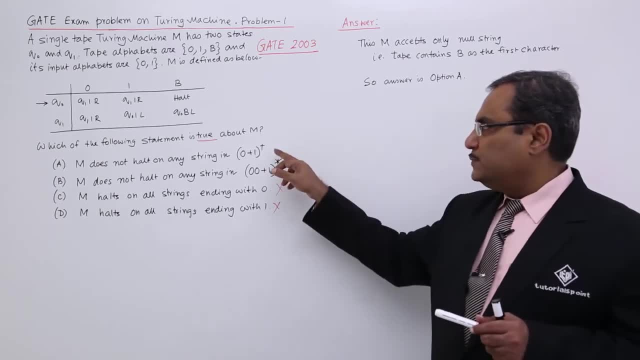 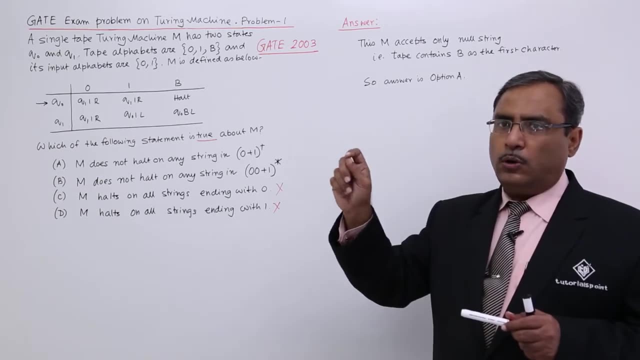 kappa, It cannot produce any null because it is plus, So it can have 0 or 1 or 0, 0, 0, 1, 1, 0, 1, 1 or other combinations of 0s and 1s, So it cannot produce any null, As it.